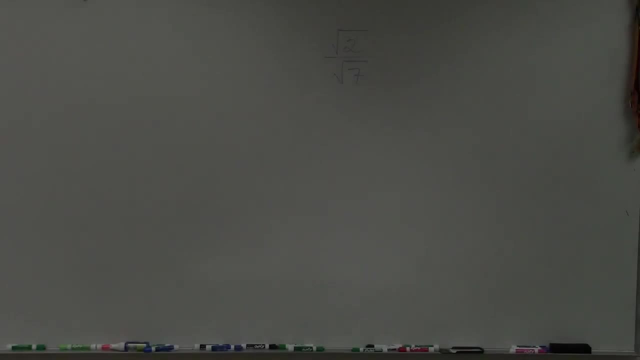 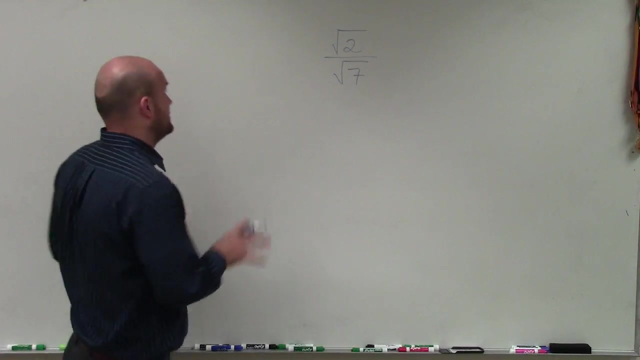 Welcome, All right. So what I'd like to do is show you how to simplify this radical expression, And we're going to use rationalizing the denominator. Now, it's very important for us to understand that when we have a radical divided by another radical, the first thing I'd say to look for 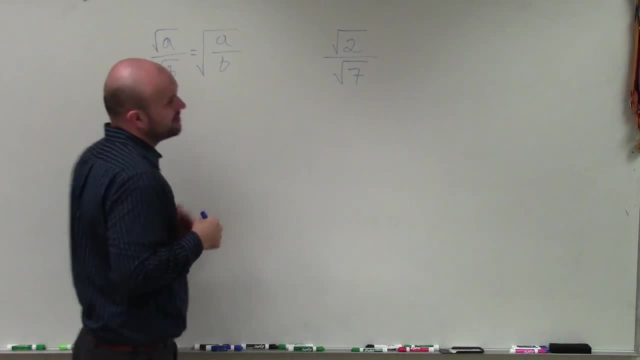 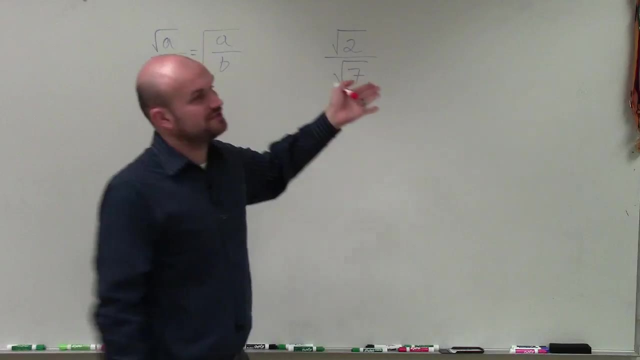 is to try to simplify our numerator and denominator by dividing them by using our properties of radicals. But the problem when we do that is we'd have the square root of 2 sevenths, which is not a perfect square number. So that's not really going to help us out. So, to simplify, 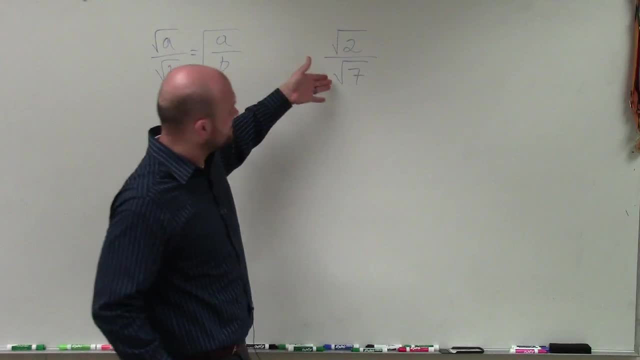 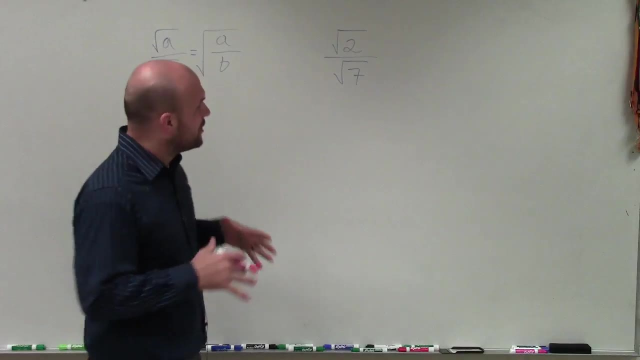 this: by rationalizing the denominator, we're going to want to get our denominator out of, or get our denominator to not have a radical in it, not have the square root of 7.. So think about this, Remember, when we're looking into taking the square root of a number we know. 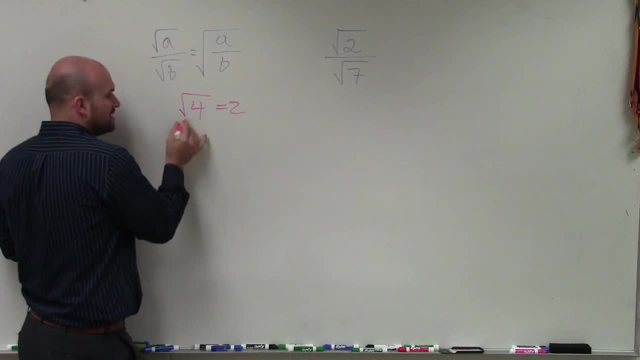 that the square root of 4 is just 2.. And why is that? Well, because we can rewrite the square root of 4 as 2 times 2.. So, basically, what we want to be able to do to undo the square root, we want to be able to take the square root of. 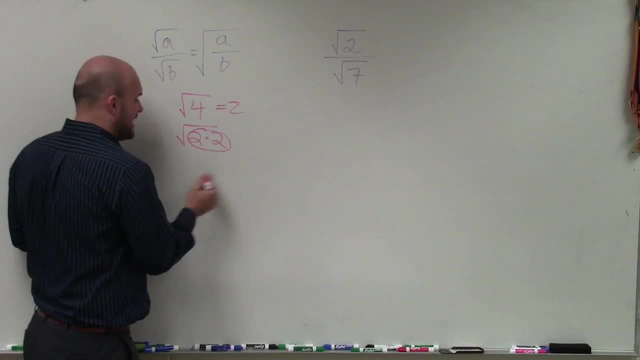 the multiplication of a number. that's by itself. And the other important thing to remember is the properties of radicals. state that when I have the square root of a number times the square root of a number number, that equals the square root of the product of those numbers. 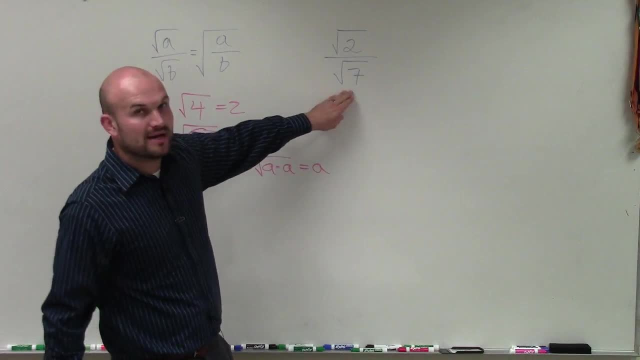 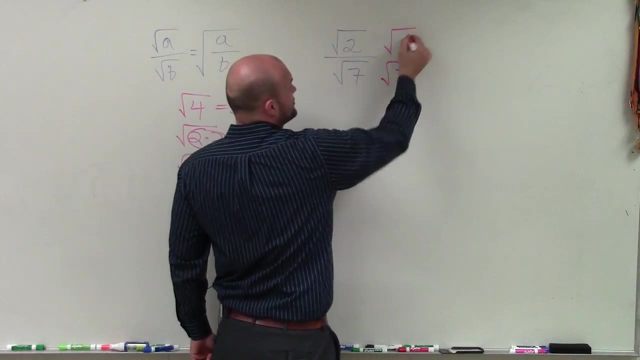 which would just be a. So the number that I'm going to want to multiply by the square root of 7, to get it just to be 7, would be the square root of 7.. And whatever I do in my denominator, I have to do immediately. 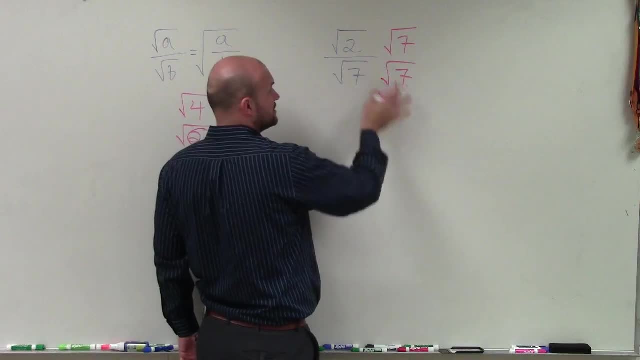 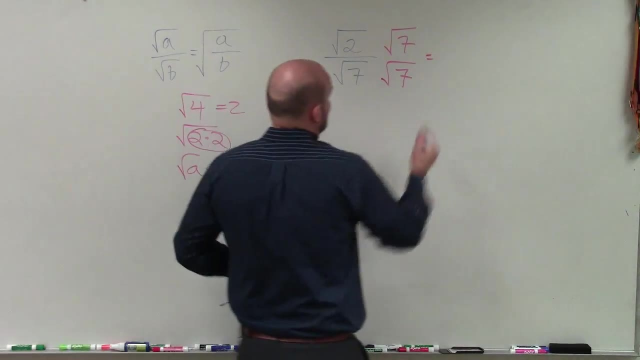 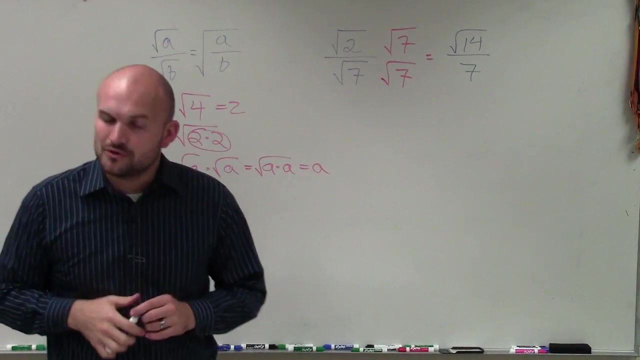 My numerator to produce an equivalent fraction. Now I can multiply these. So that's going to produce, if I put it down, that's going to produce the square root of 14 divided by 7.. So there you go, ladies and gentlemen. That is how you rationalize the denominator. 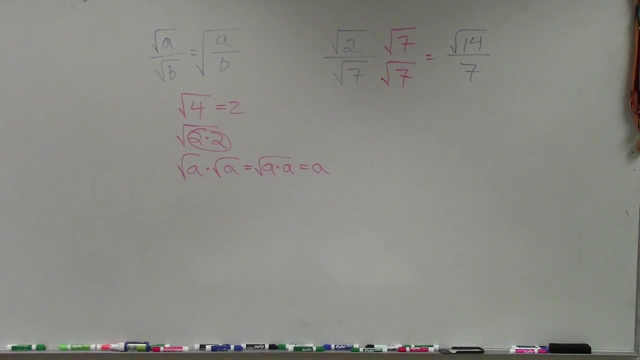 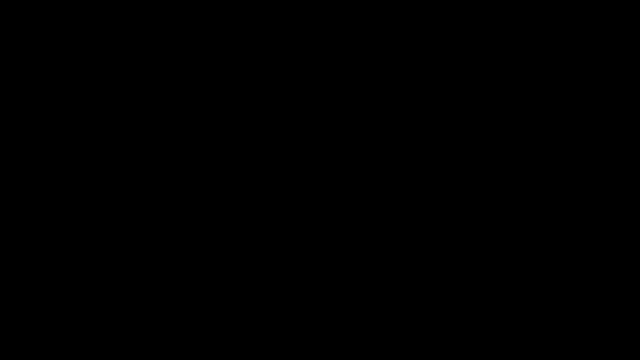 to simplify your expression, Thanks. Subtitles by the Amaraorg community.